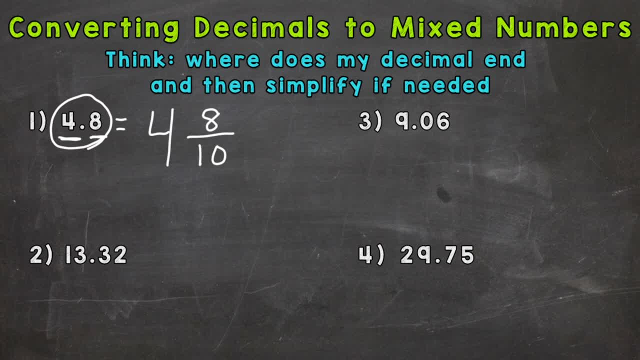 is how you would say that mixed number. They are equivalent. One's a decimal, one's a fraction. though Now, once you get to the fractional part of the mixed number, you can simplify, if it applies, and here we have a common denominator. So, if you get to the fractional part of the mixed number, 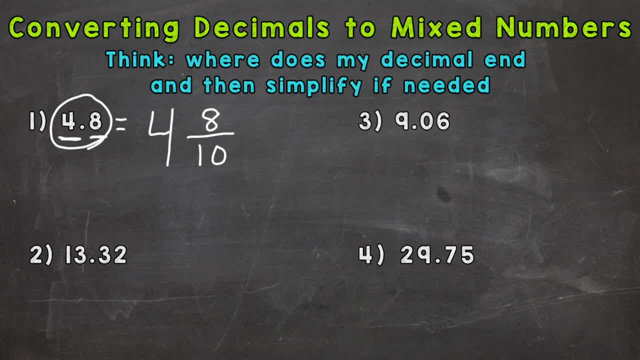 you can divide our eight and ten by two and we get to four and four-fifths. You never simplify the whole number portion of the mixed number. That stays as is and we keep it as a four. So four and four-fifths. Number two: we have thirteen. 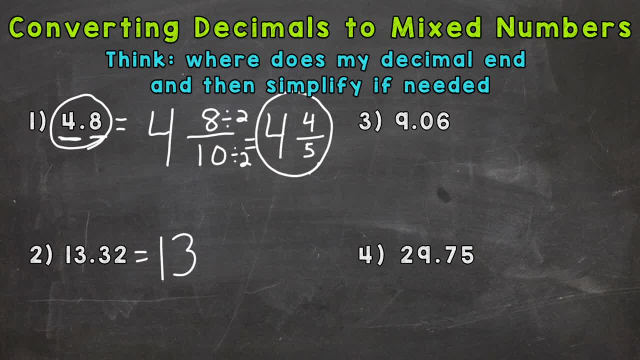 and 32 hundredths. So we always keep our whole number as is. And then where does that decimal end? Well, tenths, hundredths, it ends in the hundredths place. So that's going to be our denominator. And then whatever numbers to the right of that decimal, that's our numerator. So 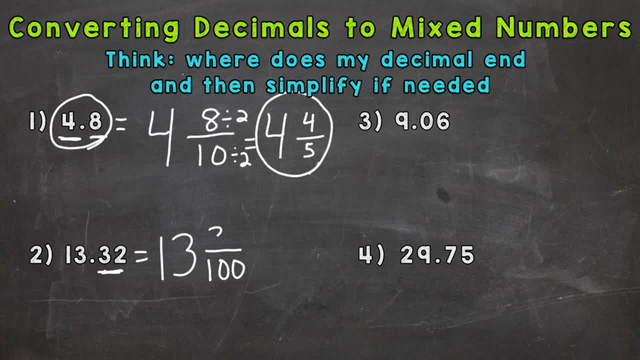 we have a 32 here, So 32 hundredths, And again, we always look to simplify when we have fractions and we keep our whole number the same. So it is a 13.. So any common factors between 32 and 100?? 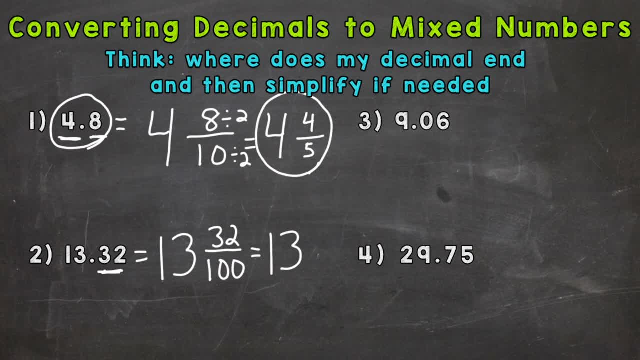 Yes, we can start breaking it down and divide each by two. They're both even Or there's a greater common factor than two. We can divide both of them by 32 hundredths. And again, we always look to simplify when we have fractions And we keep. 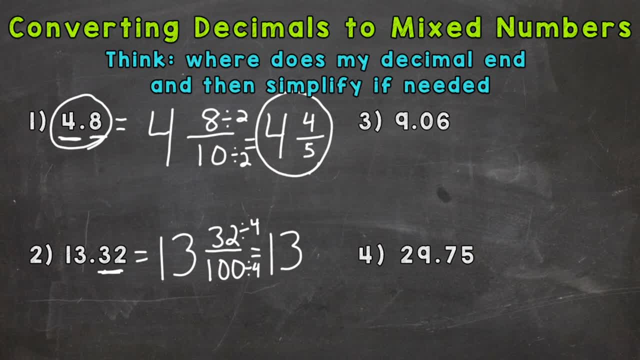 four, And we get: 32 divided by four is eight And 100 divided by four is 25.. So we get 13 and eight, twenty-fifths, Number three, we have nine and six hundredths. So nine is our whole number. Keep as. 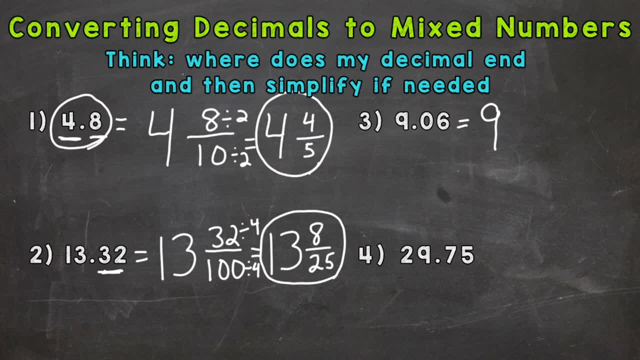 is. Let's see how far over our decimal goes. Well, it goes to the tenths, hundredths place tenths and then hundredths, So it ends in the hundredths. That's our denominator. And what numbers? to the right of the decimal? It's a six. So we have nine and six hundredths. Let's.